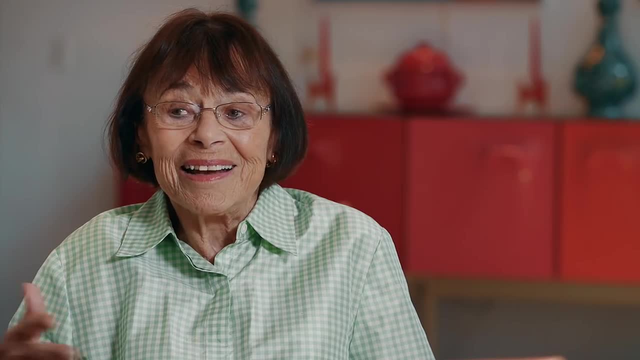 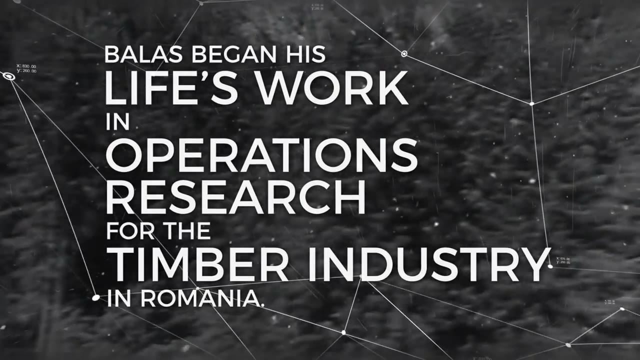 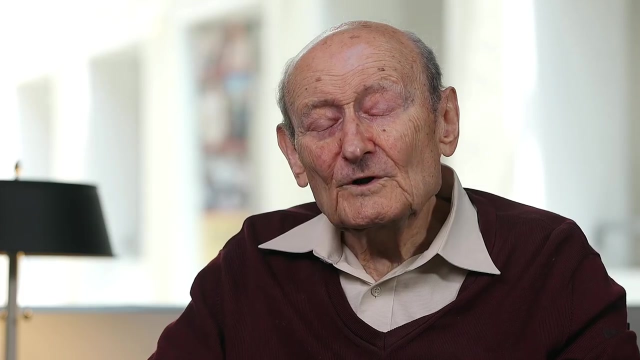 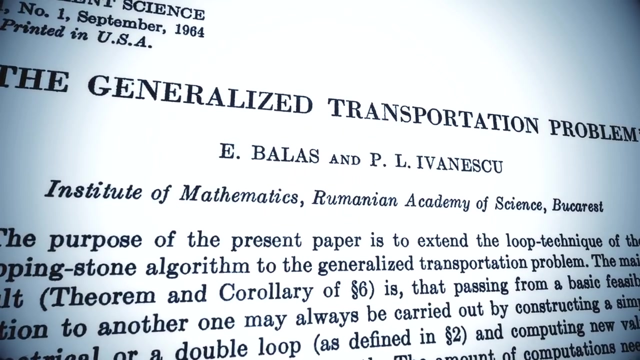 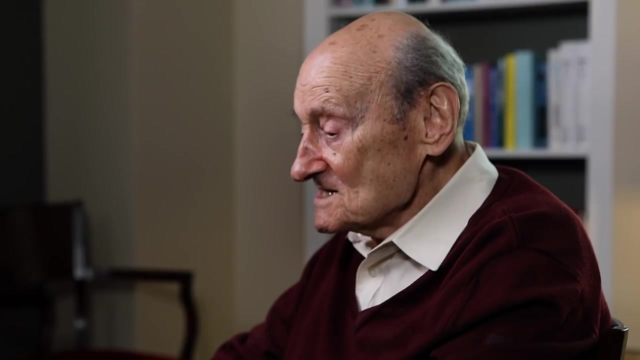 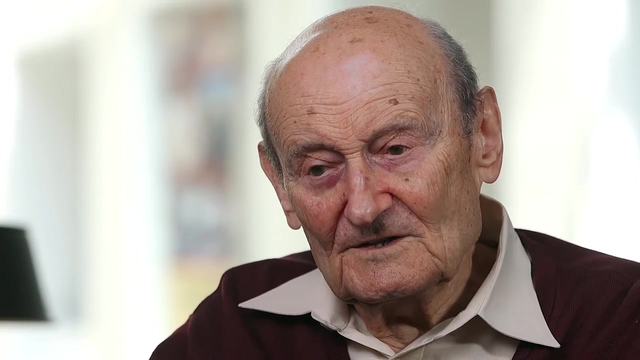 work, family and the rest of the world. My first project was joined with Peter Hammer and we worked out an optimal transportation plan for the firewood all across the country, which required the solution of a linear programming problem. In 1963, I had to solve a forestry problem. 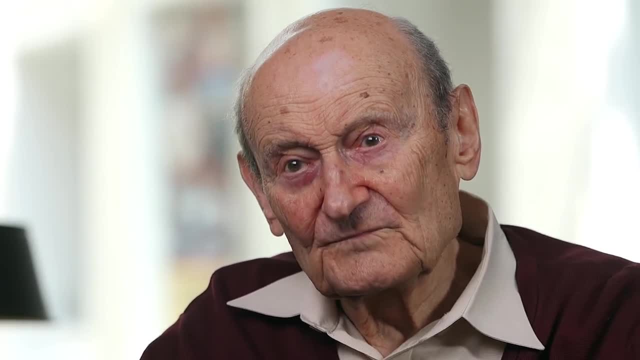 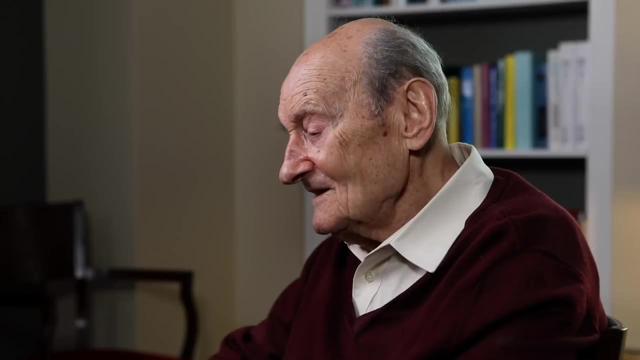 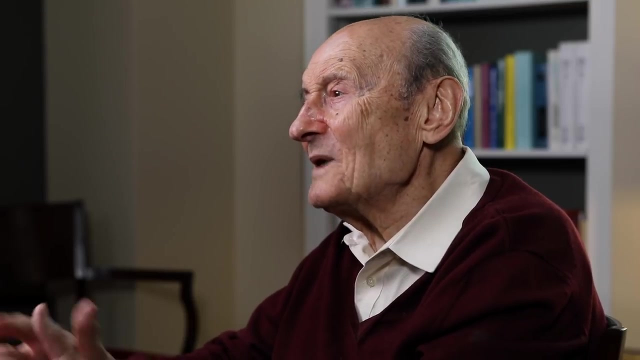 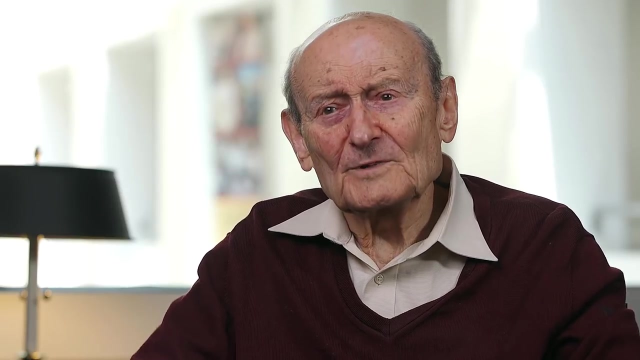 There was a plot of forests which needed a harvesting plan for the next five-year period And I formulated that as an integer programming problem: zero-one variables, yes or no variables, bivalent, we call them two-value variables. I devised my own procedure and solved the problem and presented the article first in. 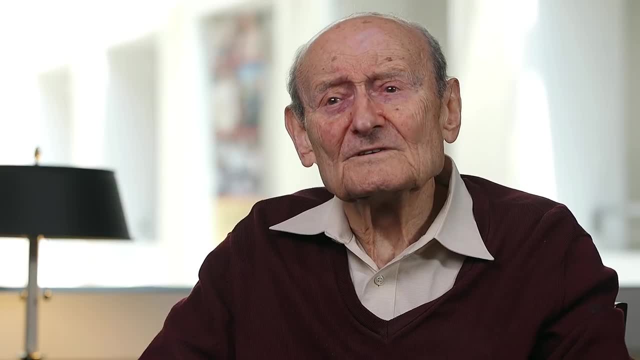 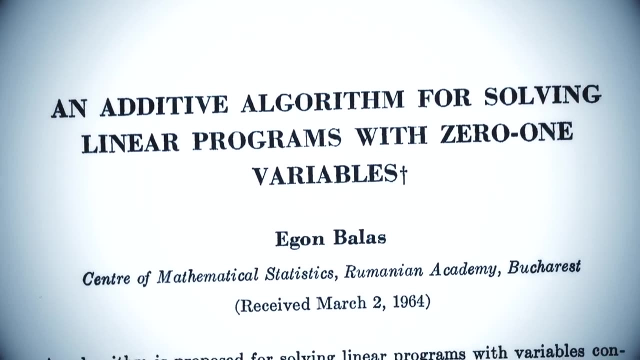 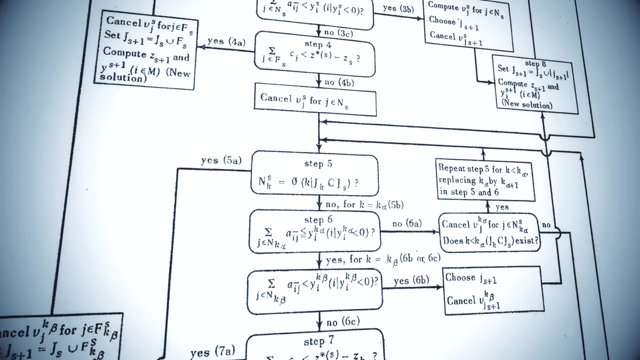 Bucharest and then sent it to the West, And that was a big hit, a big success. It's called the additive algorithm. Ultimately, it was published two years later in Operations Research And for 32 years it was the most cited article. 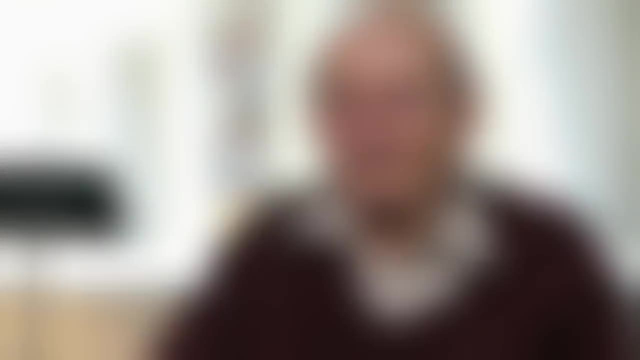 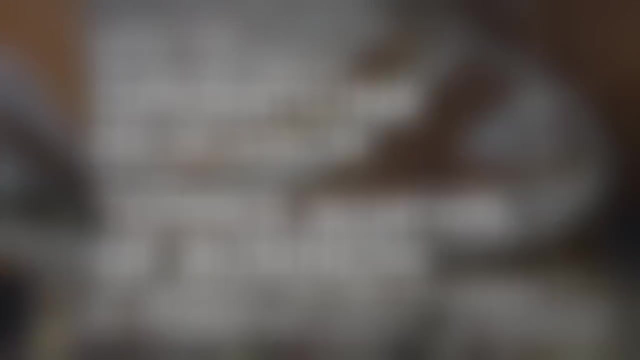 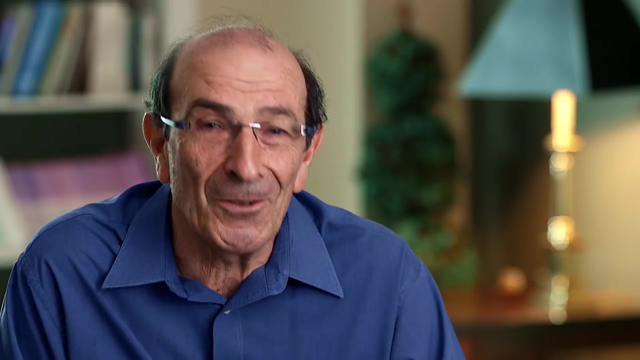 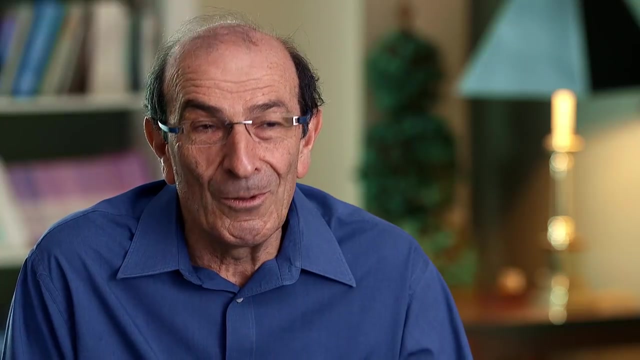 That was my status. Thank you. Step into the profession. Some people say that algorithms are now a trillion times faster than they were 30 years ago. Part of it is due to faster computers, but the bulk of it is due to better algorithms. 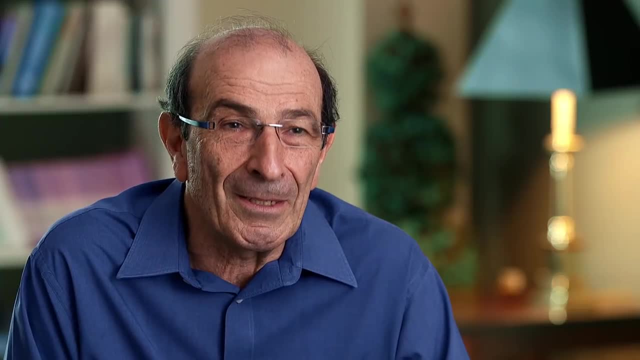 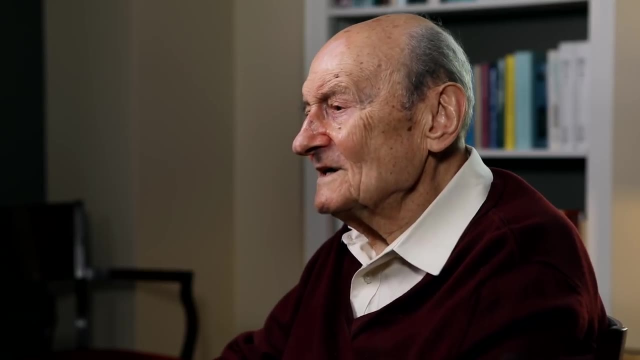 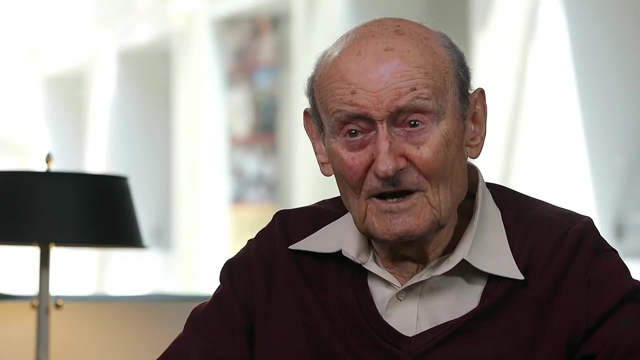 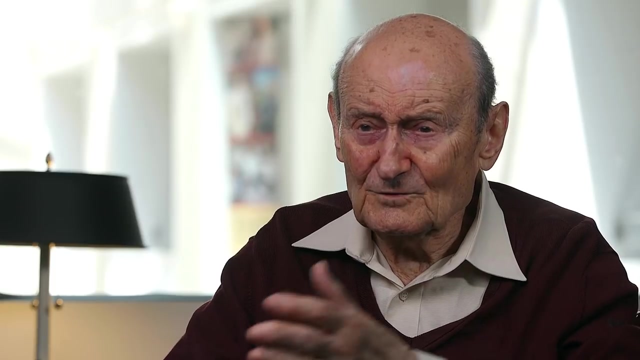 And this was pioneered by Egon Balas in the 70s. Integer programming stayed that way. a rich theory was built, but it still couldn't solve problems beyond a small number of variables for 30, 40 years, And the situation changed in this period between 1990 and 2005.. 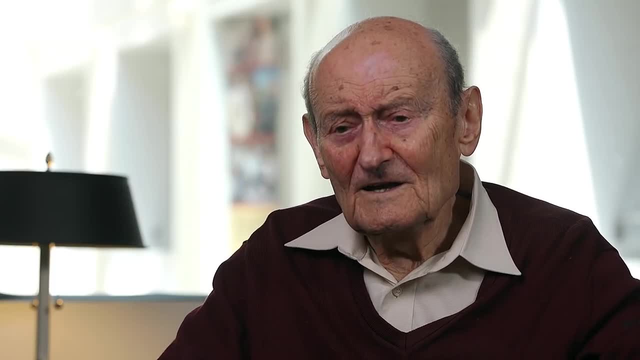 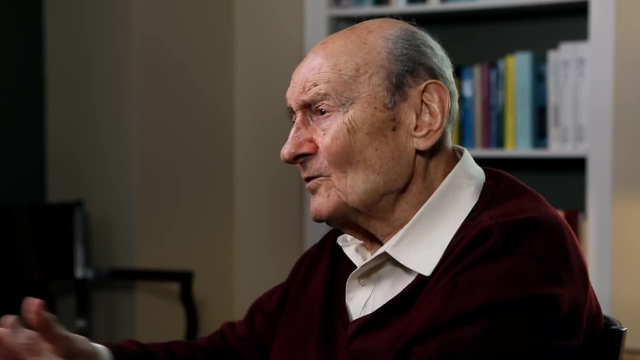 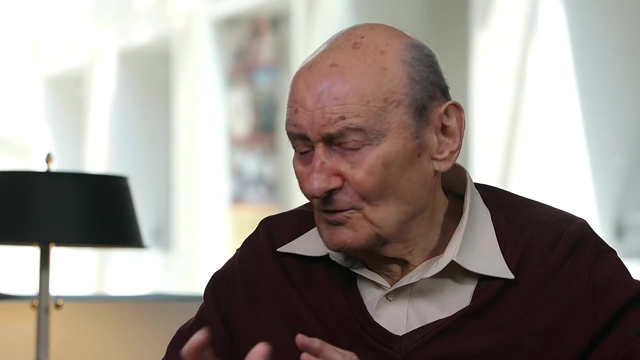 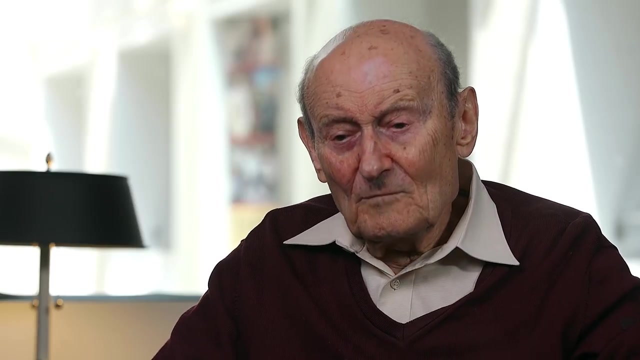 This revolution occurred in the state of the art And our work, Gerard's and mine and some others, played a crucial role in this revolution in the state of the art. So now integer programs can be solved- not all of them. There are still cases which are unsolvable in practical time. but the run-of-the-mill 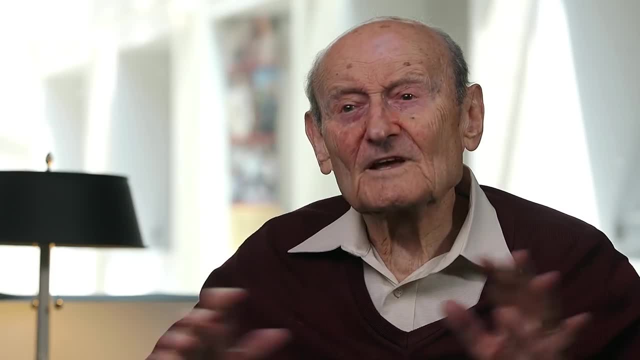 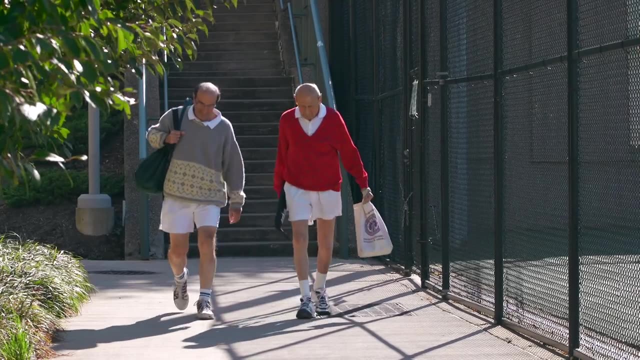 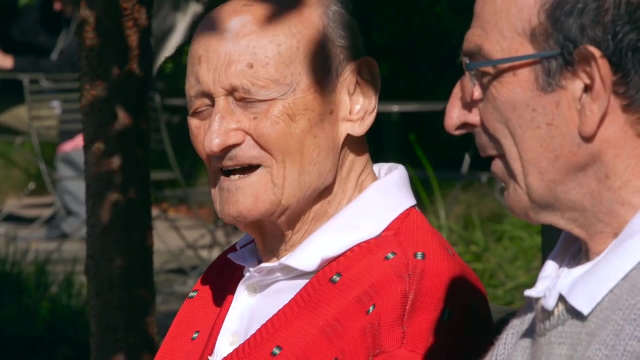 problem that you come across in practical life nowadays can be solved. This was the revolution in the state of the art of the integer programming. We talk a lot. we are very good friends, you know. it's always a pleasure to bounce off ideas. 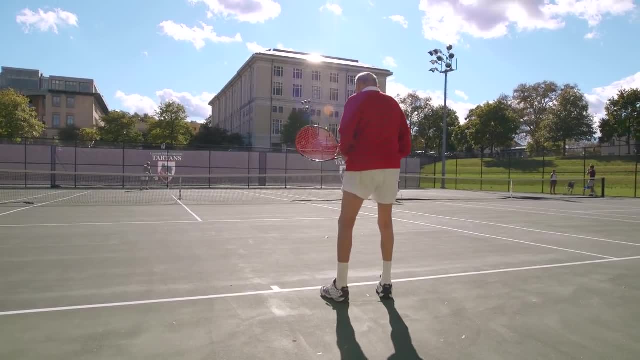 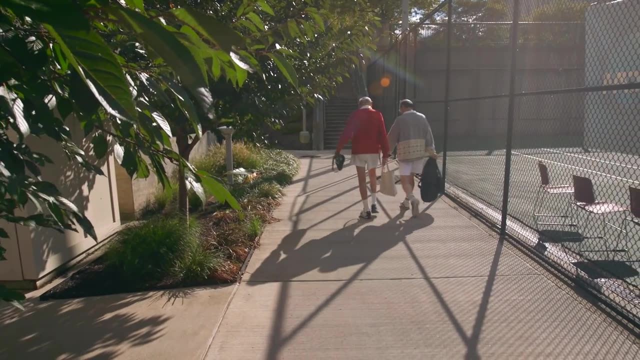 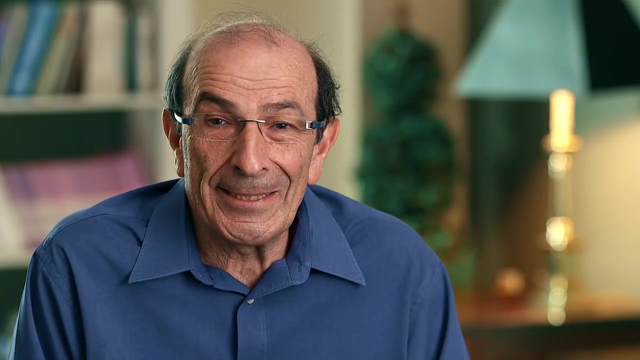 On Wednesday evenings we play tennis. we've been doing this at least 20 years, probably more. He's done so much for me. I'm just so grateful that I have such a friend. He has this very independent way of thinking, very unique way of thinking. so you know. 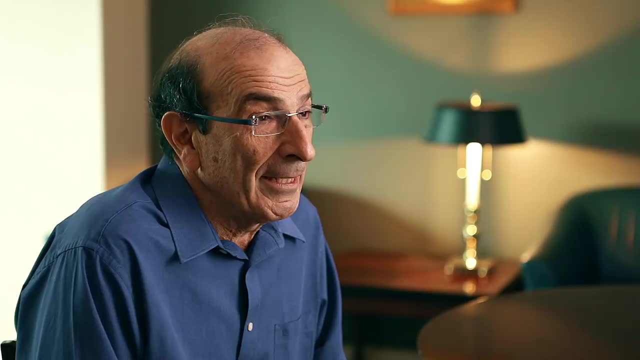 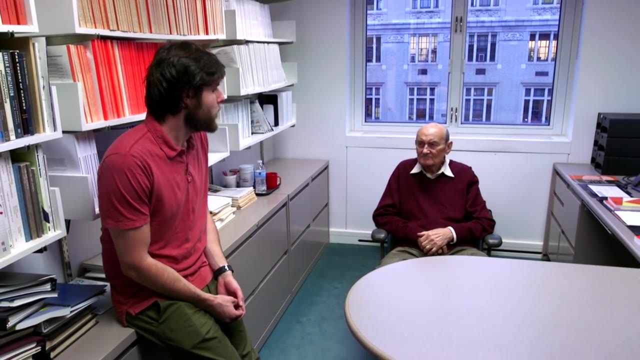 that makes him a great researcher, because you know he doesn't think like others would. Do you have an example in mind? Yes, so this is an example. Working with Dr Balish is it's an honor and a privilege. 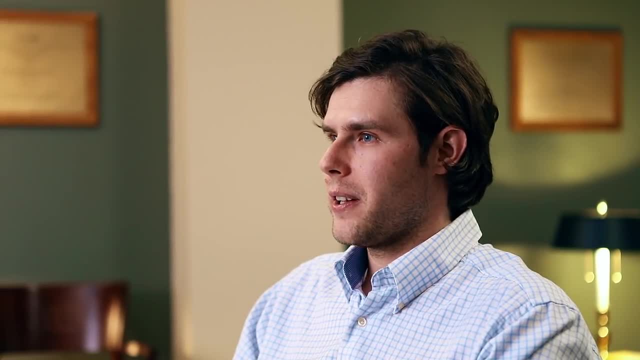 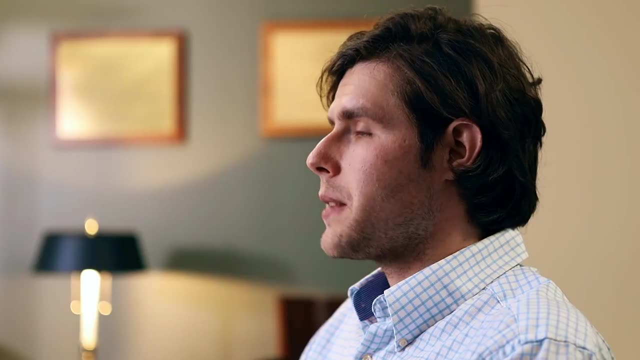 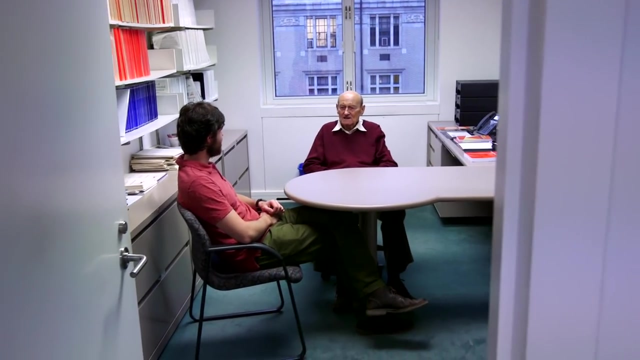 He's really really good at forming the story that is told. Given the same kind of data, you can tell different types of stories- And he's very good at seeing the bigger picture. He wants to make a real practical impact, Meaning that he won't work on theoretical questions if there are no practical impacts. 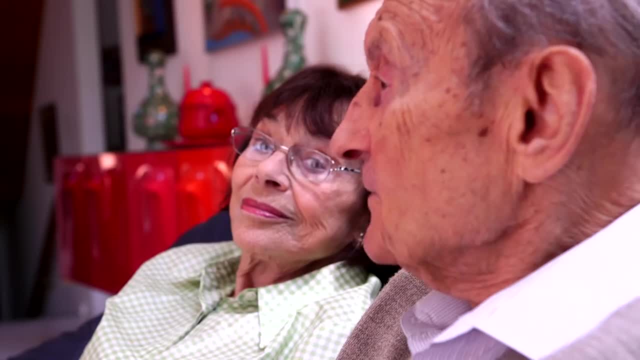 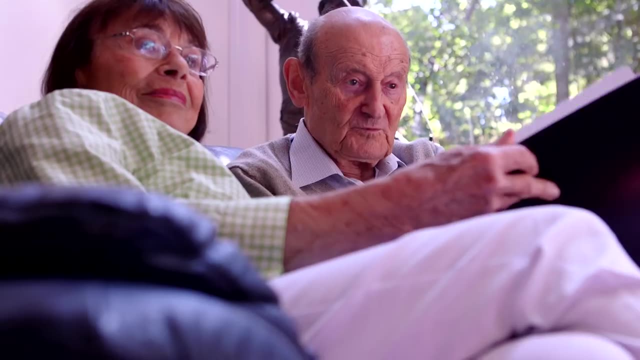 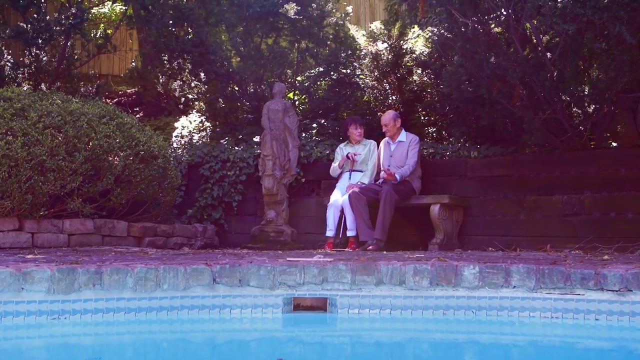 that can be made from that in the future that he sees His gift is intellectual capability, concentration, discipline. What he has to do, he would do that, So he is very focused. He is not interested in what is happening. He didn't know about ladies. 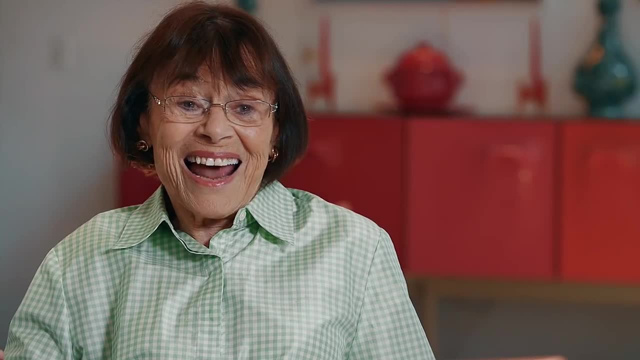 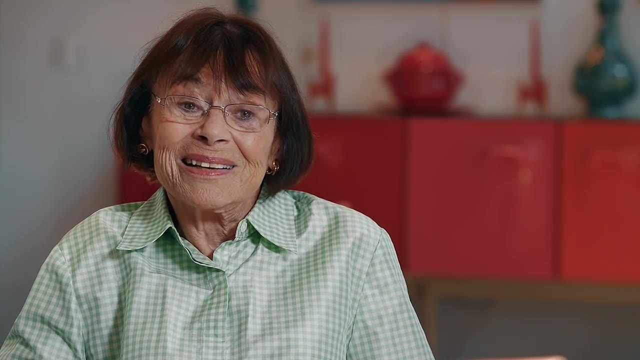 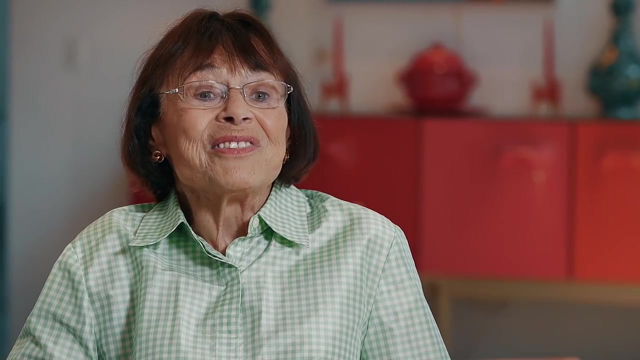 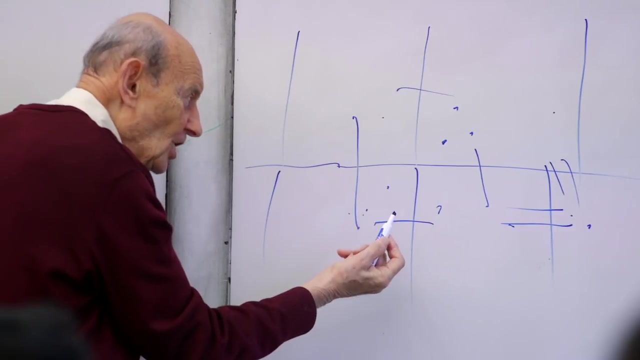 He didn't know about Lady Gaga until last year, or anybody. He is very, very focused in his work, which is good, because this is how people achieve something. Having Dr Balish on the Tepper faculty, I think, has and will continue to influence. 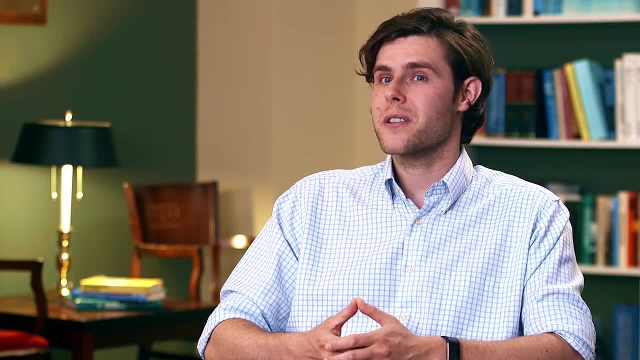 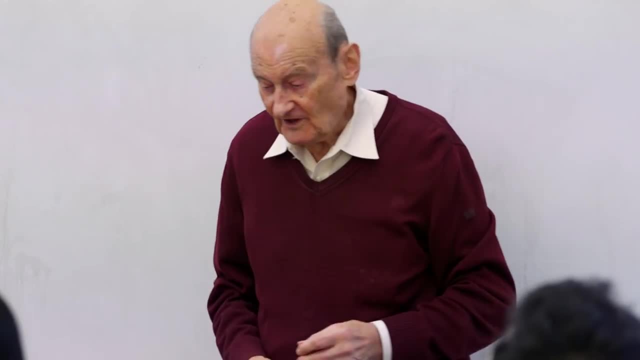 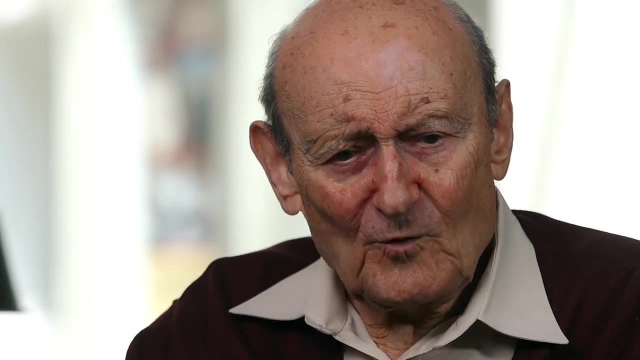 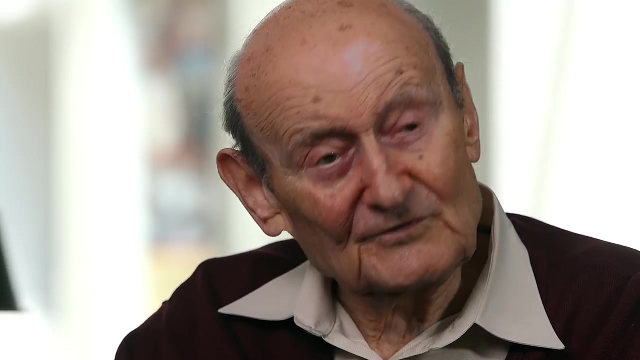 the path that Tepper takes for generations to come. Most people do a job which after a while becomes boring and work becomes a burden, And so retirement is a very wise institution and necessary. But some people who are very lucky- I consider myself among those- have a job which they